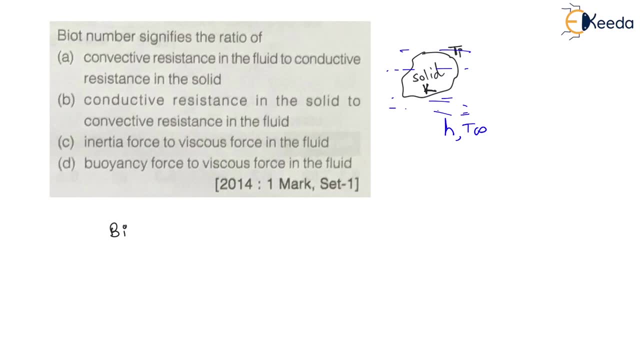 K is the thermal conductivity of solid. And let us assume the initial temperature of solid object is more than surrounding fluid temperature. Therefore, my dear students, because of this temperature difference, can I say this solid object will continuously lose heat to the surrounding by convection. 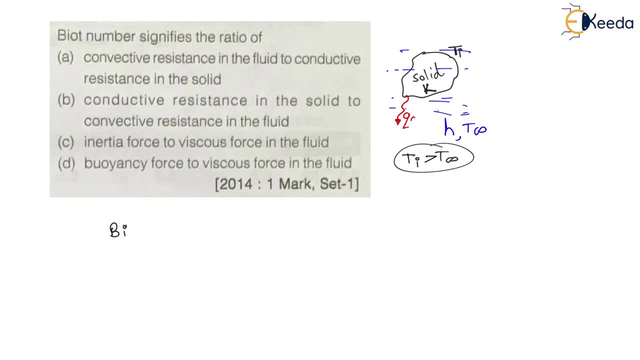 Therefore, the solid object will continuously lose heat to the surrounding by convection, And slowly, slowly, the temperature of solid object goes on decreasing. Right Now, my dear students, this Bayard number is defined as it is: H? L divided by K of solid. 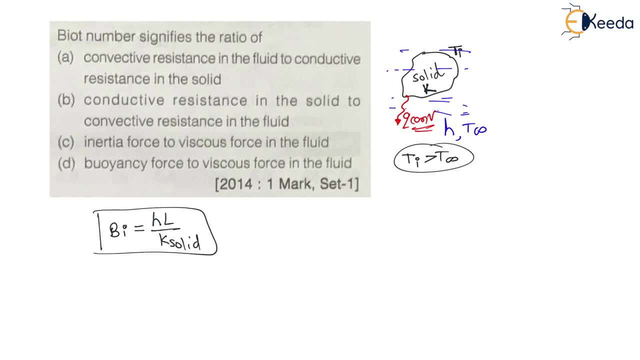 Right, It is for solid object. Thermal conductivity is for solid object. You might have learned about Nusselt number, which is used in convection, Right. This Nusselt number is nothing but H, L divided by K of fluid, and it is used in convection. 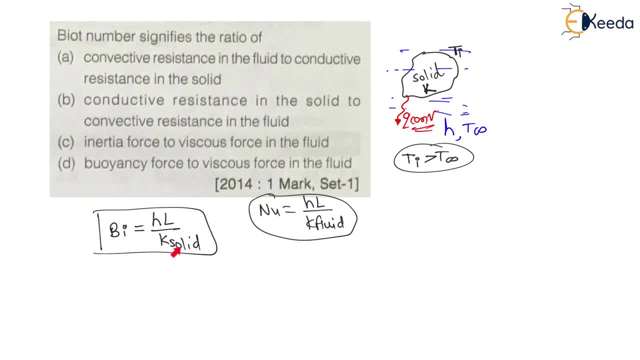 Right, That is in fluids. But Bayard number is H? L divided by K of solid. This is very important, Right? So, my dear students now here, Bayard number is H? L divided by K of solid, where H is convective heat transcoefficient between solid body and the surrounding fluid. 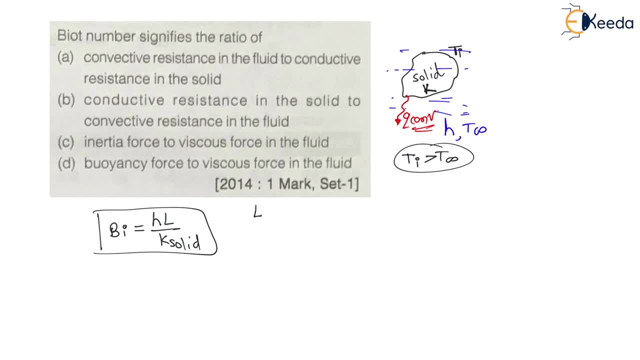 L is a characteristic dimension Here. this L is characteristic dimension which is nothing but volume of the body. They have a surface area of the body in contact with the surrounding fluid. They have a surface area in contact with the surrounding fluid Right Volume divided by surface area. this is characteristic dimension. 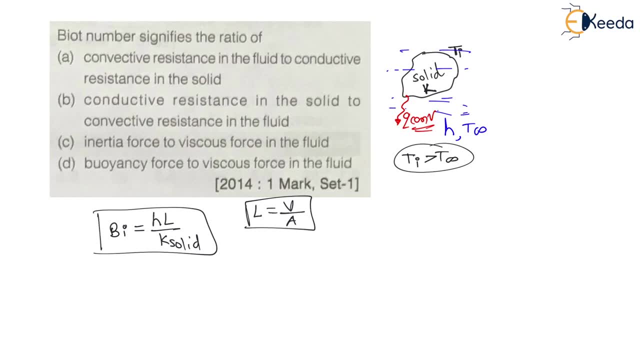 And K is a thermal conductivity of this solid body, Right. So, my dear students, can I write this Bayard number as? let us write this Now: H, L divided by k of solid Right Now. if I multiply this with area and divide with area, then it is absolutely fine. 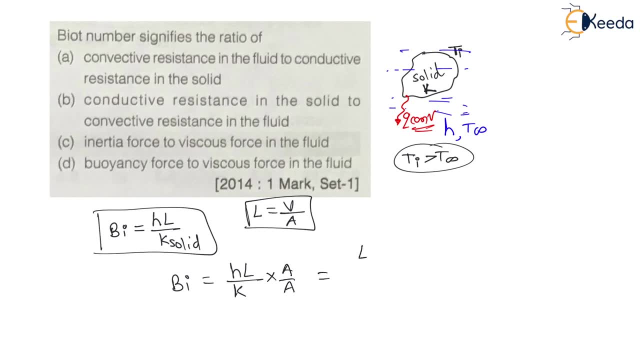 Again. can I write that it is as L divided by K a, L divided by K a. this term, This term is even This L, this K and denominator A And this HA. I will take to the denominator of this. Therefore, it will become 1 upon HA. 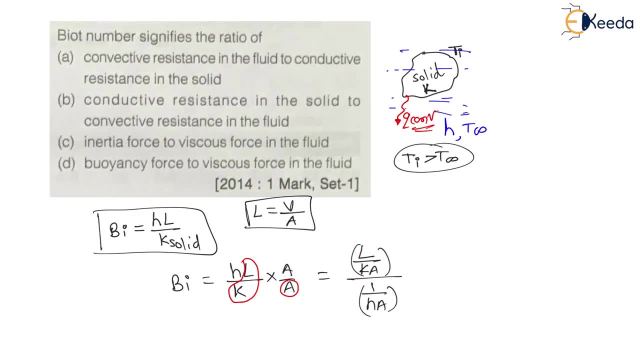 And my dear students, L divided by KA. KA is the thermal conductivity of solid. Therefore, this L divided by KA in conduction topic, in plane slab topic, we have seen this is the conduction resistance of solid And therefore we can say this: L divided by KA is conduction resistance R conduction of solid. 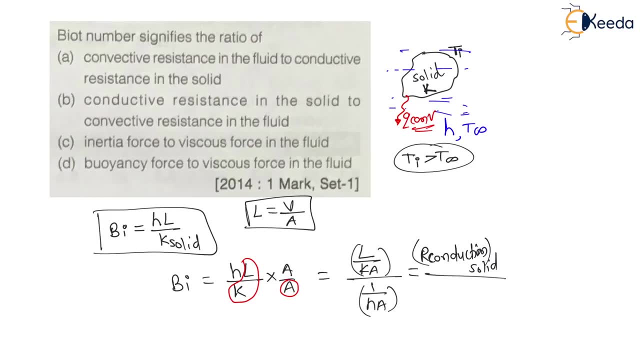 Of solid right, It is R conduction of solid divided by. Again, in convection topic, we have seen: 1 upon HA is convection resistance. Therefore it is R convection. Therefore, my dear students, the definition of biot number is: 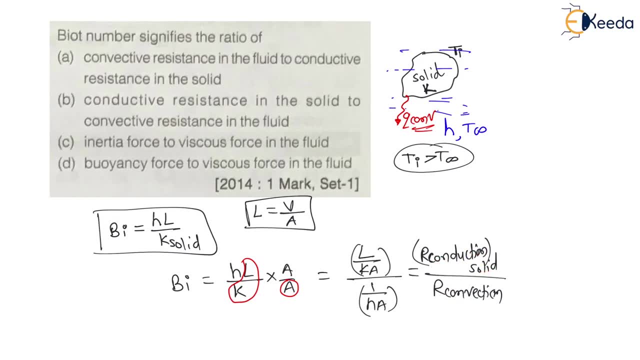 it is a conduction resistance of solid divided by convection resistance of surrounding fluid. So the same biot number, The same biot number we can define, as now. let us understand The same biot number we can define, as this biot number is nothing but. 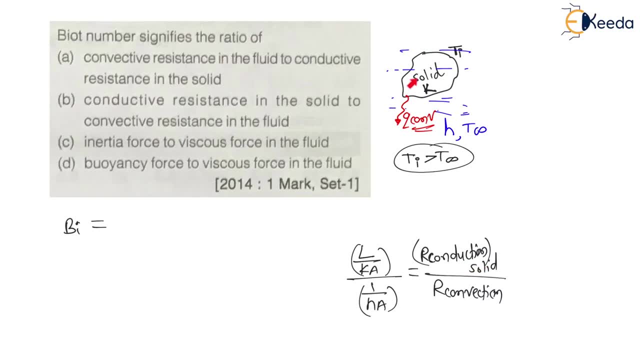 Now here it is a conduction resistance of solid Means. we can say it is a internal conduction resistance of this solid Right. It is a internal conduction resistance of solid divided by. It is a convection resistance, And convection resistance is external to the solid. 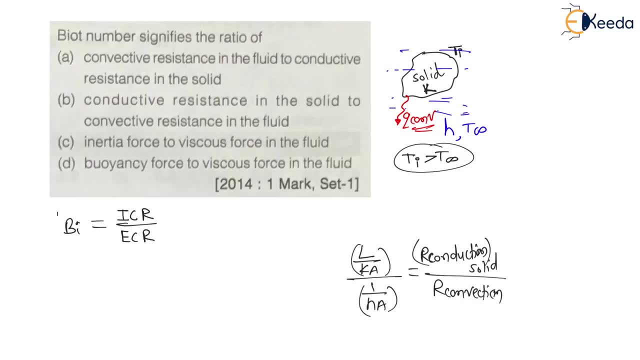 Therefore, we can define external convection resistance. Therefore, my dear students, the biot number is defined as internal conduction resistance of solid divided by external convection resistance. This is the basic definition of biot number. Now here, whenever this biot number value is less than 0.1,. 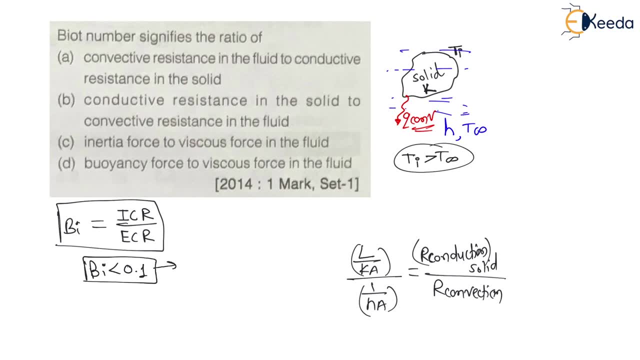 then the problem is called lumped heat capacity analysis, Then the problem is called lumped capacity analysis or lumped analysis problem. Lumped capacity heat analysis or lumped analysis problem. And, my dear students, whenever biot number is very, very less, that is, 0.1.. 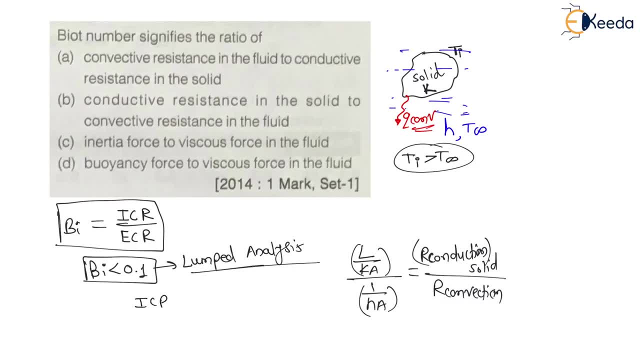 That means we can say: the internal conduction resistance is very, very less as compared to external convection resistance. Right, Therefore, simply, we can say: whenever it is a lumped analysis, then biot number is very less, Then internal conduction resistance is very less as compared to external convection resistance. 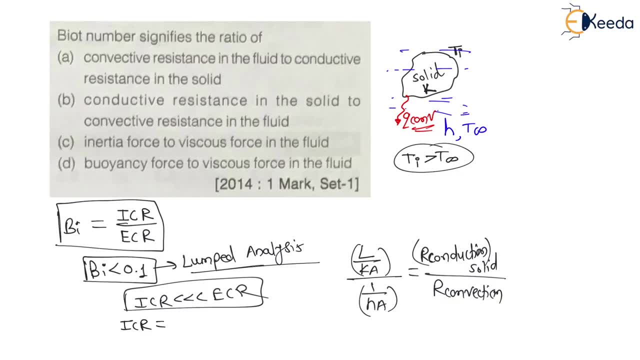 Therefore, simply, we can ignore this internal conduction resistance. This internal conduction resistance is almost negligible, Almost negligible. Therefore, my dear students, the definition of lumped analysis is nothing but the biot number is very less, less than 0.1, and the internal conduction resistance is negligible. 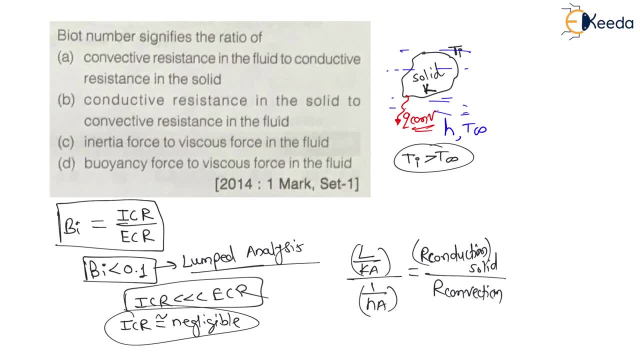 Then it is called lumped analysis. Now, on these all concepts, they can ask you any question Right Now. let us understand here one by one. Now, very first question is: the biot number signifies the ratio of. It is a conduction resistance of solid divided by convection resistance. 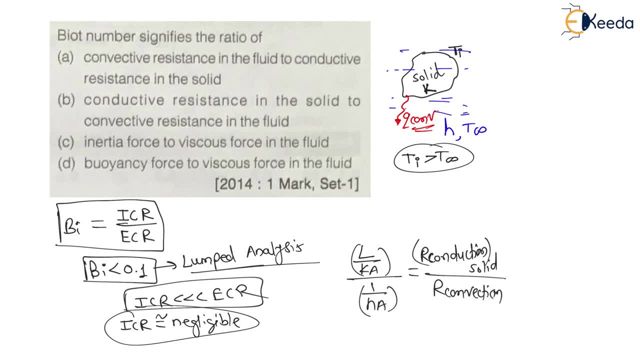 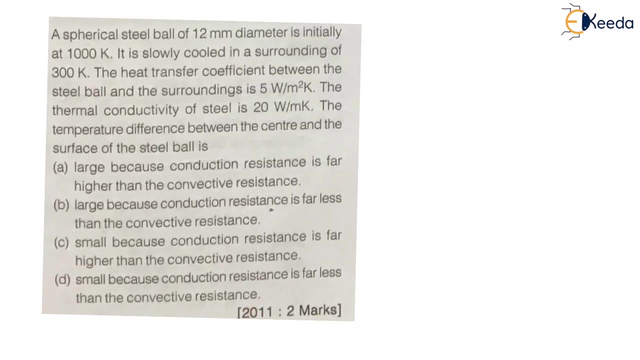 So conduction resistance in solid, So the convection resistance in fluid. Convection resistance is always in fluid. Therefore, for this question, option B will be the correct choice. Now let us look at the second question. Now, the second question, which was asked in GATE 2011 for two marks, is based on biot number again. 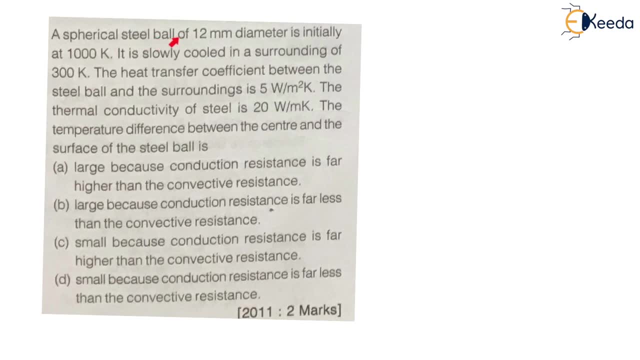 So let us understand the question. The question is a spherical steel ball. Now, my dear students, they have given spherical steel ball Right Of 12 mm diameter. So here I can say, let us draw this pair. Let us say this is a ball. 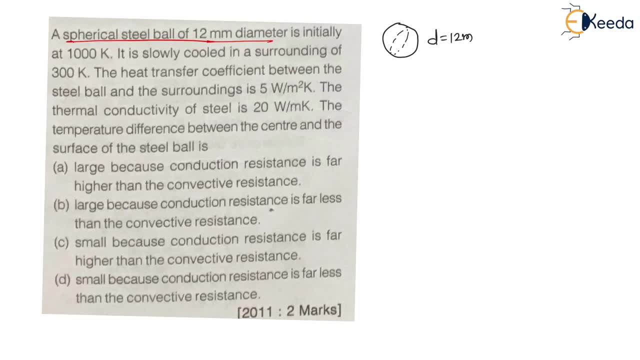 It is spherical Right, Having diameter 12 mm. Therefore, can I say diameter is equal to 12 into 10, to the power minus 3 meter Right Now is initially at 1000 Kelvin. Now, initial temperature of this ball Ti is nothing but 1000 Kelvin. 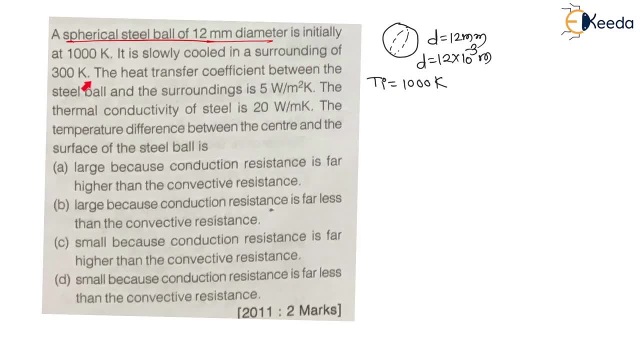 Then it is slowly cooled in a surrounding of 300 Kelvin. Now surrounding temperature which is T infinity is given 300 Kelvin, Then the heat transfer Coefficient between the steel ball and the surrounding is 5 watt per meter square Kelvin. 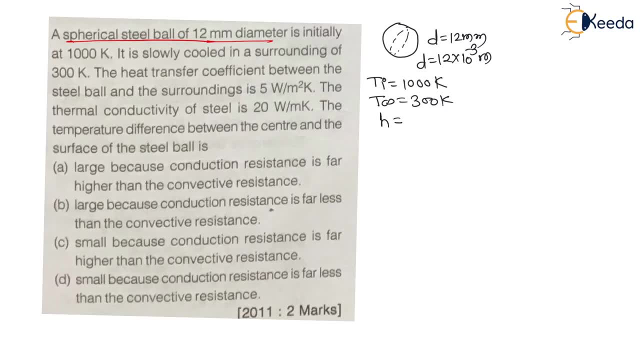 Now it is. heat transfer coefficient means h. Between the ball and surrounding is h. It is 5 watt per meter square Kelvin. Right Then, the thermal conductivity of steel is 20 watt per meter Kelvin. Therefore it is K value is 20 watt per meter Kelvin. 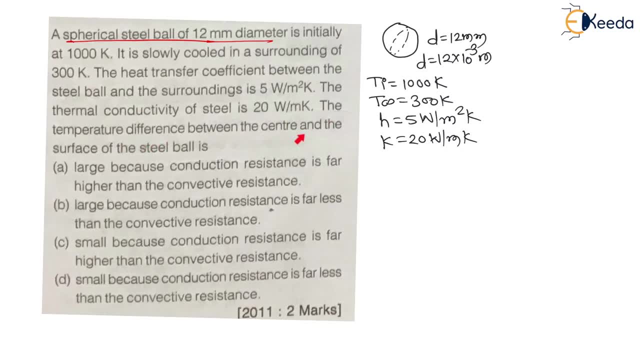 After that, the temperature difference between the center and the surface of the steel ball is Now water, this steel ball. we have to find this temperature difference between center and the surface. this temperature difference we have to find now. let us understand here. first of all, let us check. 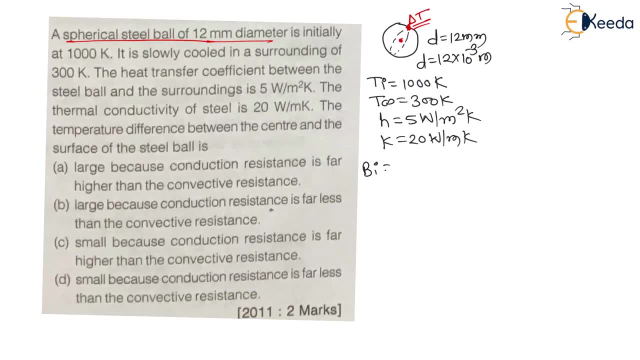 the biot number. now, my dear students, biot number is nothing but biot. number is hl divided by k red, where l is volume divided by surface area. therefore, this l can be calculated as volume divided by surface area. volume of sphere is 4 by 3 pi r cube. surface area is 4 pi r square. 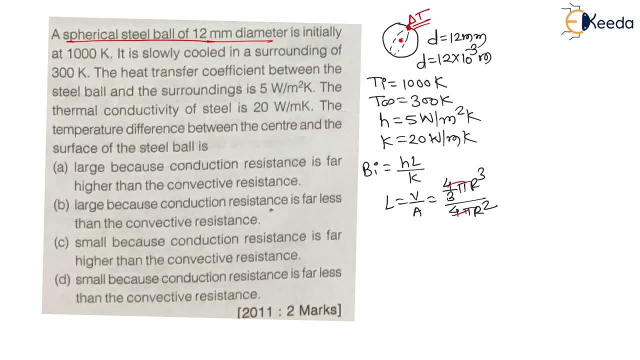 therefore, here, 4 pi, 4 pi and r square. r square will get cancelled, it will remain r by 3. this characteristic dimension will remain r by 3, which is nothing but d by 6 red. so, my dear students, let us put this l as d by 6 over here. then this biot number will become h, d by 6 into k. so let us put. 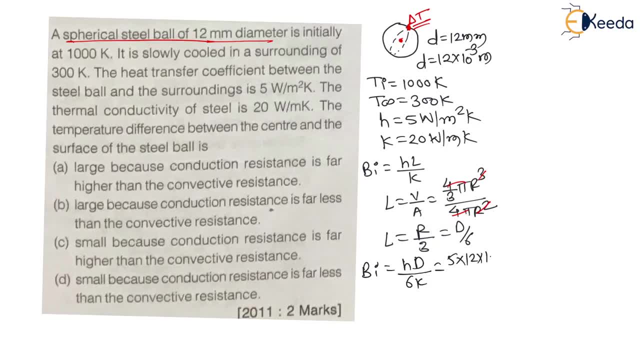 the values. h is given 5. diameter is 12 into 10. to the power minus 3 divided by 6. into thermal conductivity is given 20. if i find this biot number i will get. biot number is equal to 5 into 10, to the power minus 4 which. 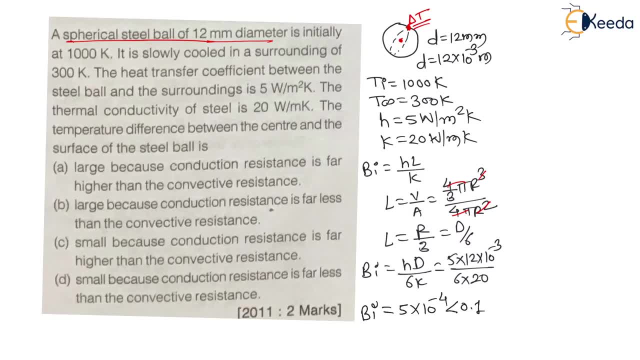 is very, very less, and again we can say it is less than 0.1. therefore, my dear students, for this question, the lumped heat analysis is valid. right, for this question, the lumped heat analysis is valid and as biot number is very, very less, the definition of biot number: just now we have seen: 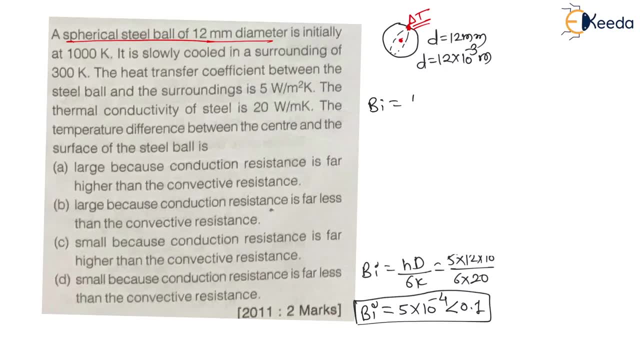 the biot number is nothing. but this biot number is nothing but internal conduction resistance of solid divided by external convection resistance. therefore, as biot number is very less, we can say: this internal conduction resistance offered by solid is very, very less as compared to external convection resistance. now, as there is no resistance, 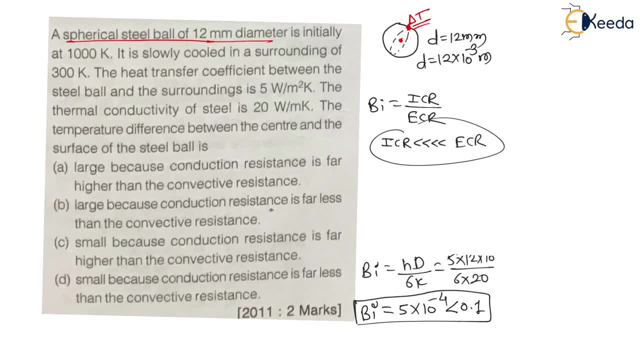 internally. therefore, the heat transfer will be maximum, thereby normalizing the temperature of body same at each and every location. whenever internal conduction resistance is very, very small, then the at each and every temperature location the temperature of body will be same because the resistance is very small. therefore, heat transfer is very high. heat transfer will be very 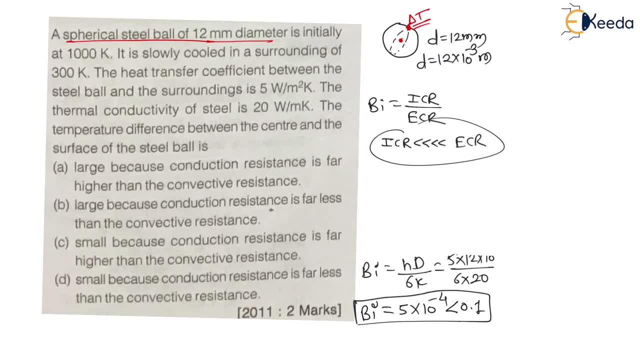 high, therefore normalizing the temperature at each and every location. therefore, at each and every location, the temperature will be same. therefore, change in temperature within body will be approximately equal to zero, right. therefore, the temperature difference between center and surface will be very small. right now, let us understand. here they are asking the temperature difference. 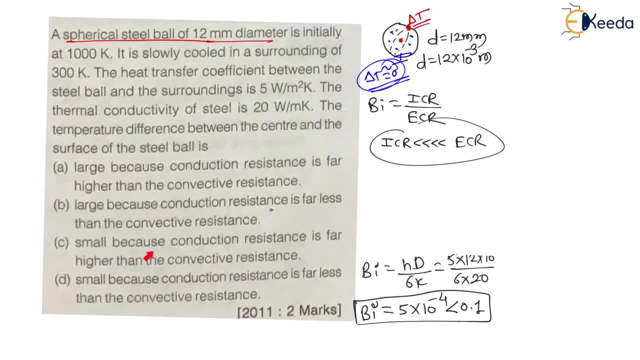 between the center and the surface of the steel ball is small because conduction resistance is far higher. sorry, it is not the correct conduction. they are saying conduction resistance is far higher. no, conduction resistance is far lesser now here. small because conduction resistance is far less than the convection resistance. yes, exactly, option b will. 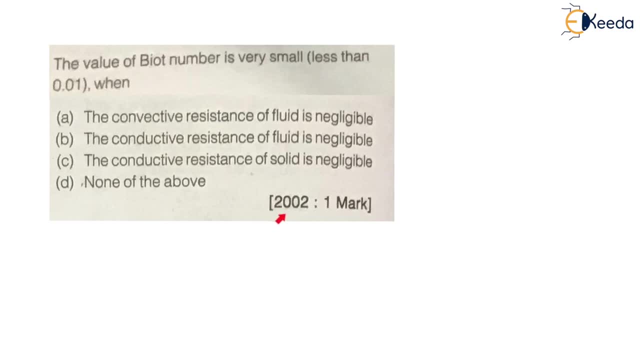 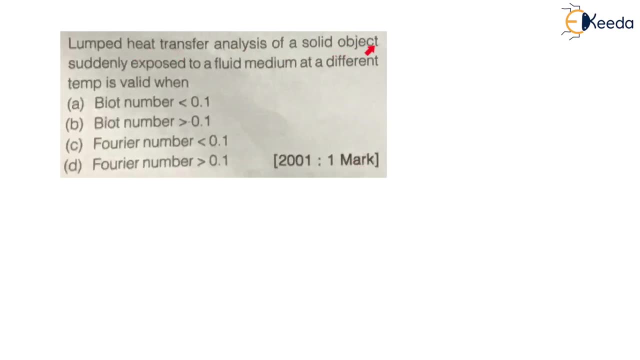 is the lumped heat transfer analysis of a solid object suddenly exposed to the fluid medium at a different temperature is valid, when now they are saying the lumped heat analysis is valid when the biot number is less than 0.1? just now we have seen. therefore, option a will be the correct choice. 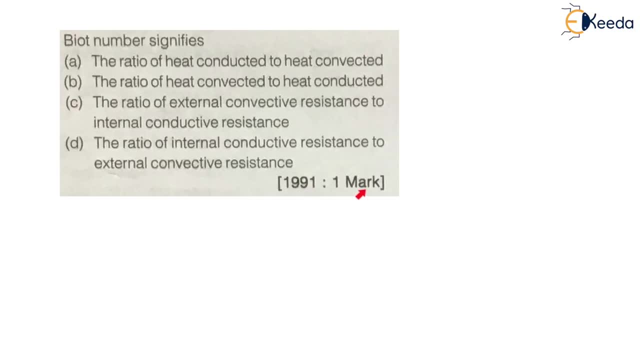 again very simple: from gate 1991 for one mark, biot number signifies we have seen the biot number. biot number is nothing but internal conduction resistance of solid divided by external convection resistance of fluid right. so let us check the option: the ratio of internal conduction resistance. 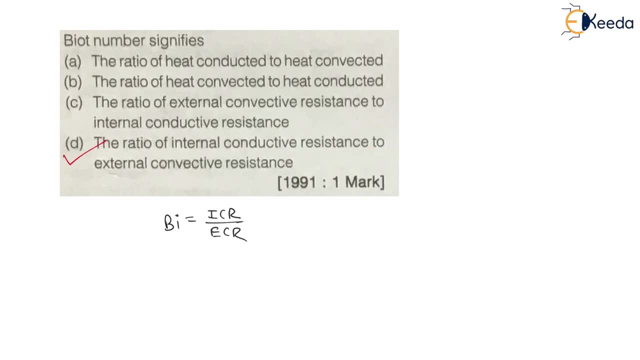 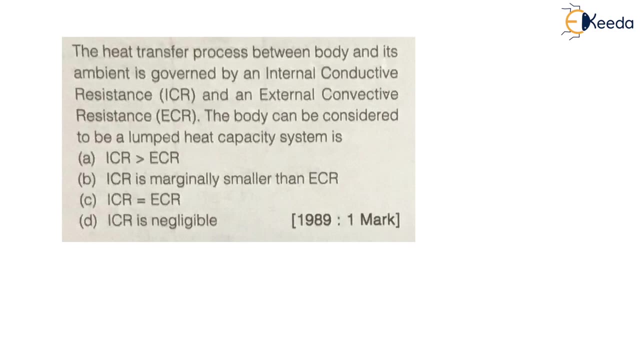 to the external convection resistance. therefore, for this question option d will be the correct choice. again, the next question from gate 1989, for one mark. again very simple question, again repeating, on the biot number. only the heat transfer process between a body and its ambient is governed by an.